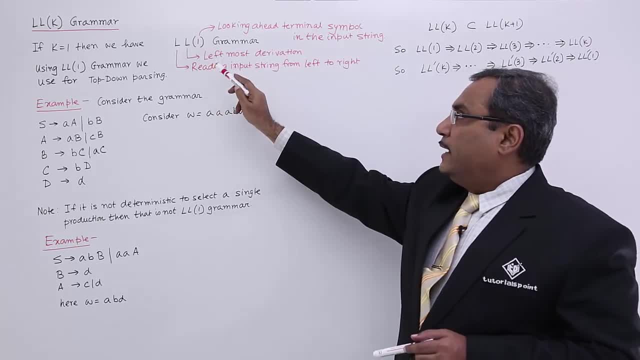 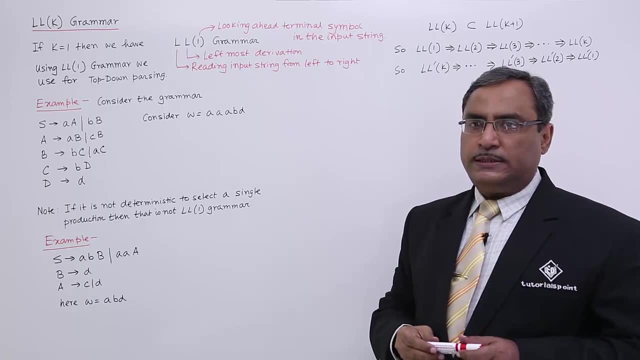 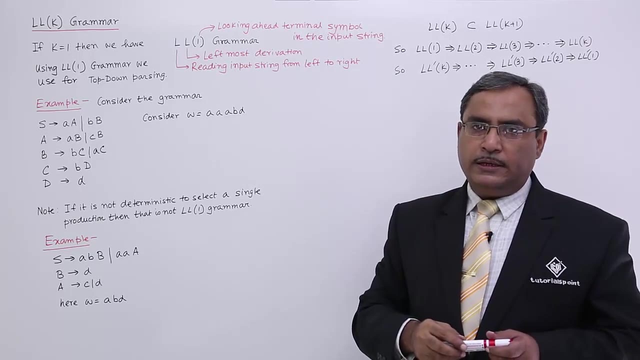 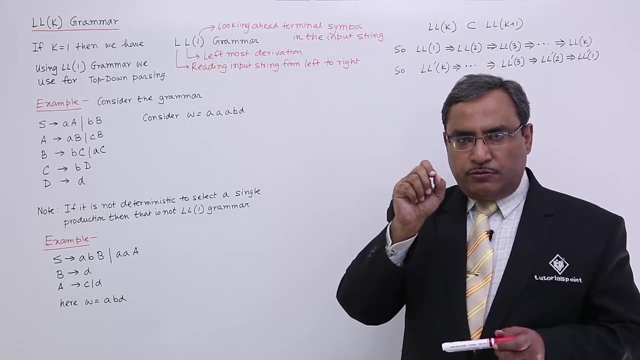 And what about the second L? The second L will indicate that the leftmost derivation will be used in the sentential forms. So leftmost derivation means in the sentential form the leftmost non-terminal will be deduced at first. So that is my leftmost derivation. And this 1 means in the input string. we shall read one symbol at a time. 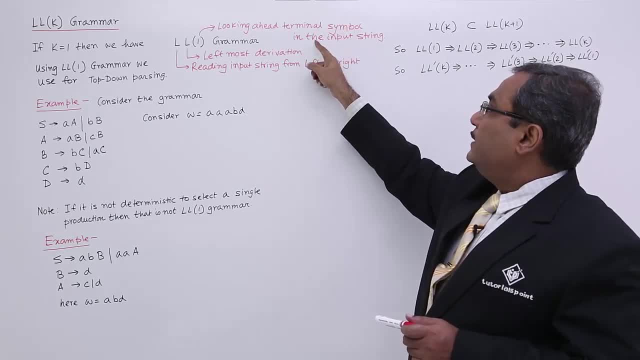 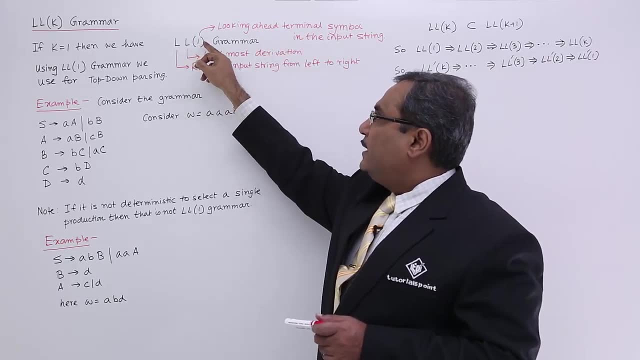 So looking ahead terminals In the input string. here it is 1.. So looking ahead for one terminal symbol in the input string. if it is LLK, then looking ahead K terminal symbols from the input string. So that is our LLK or LL1, whatever. 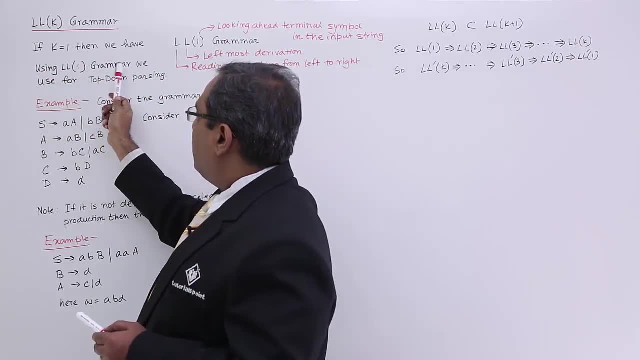 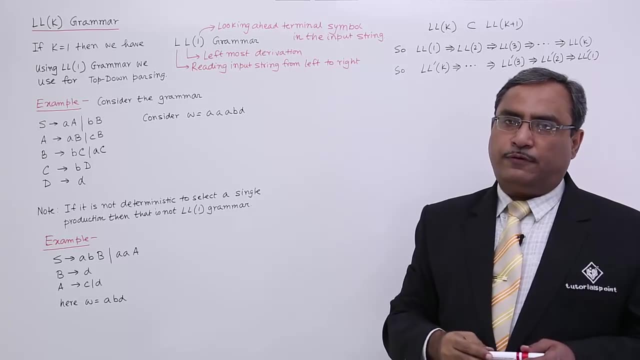 If K is equal to 1, then we have this. Okay. LL1 grammar we use for top-down parsing. So LL grammar we will be using for top-down parsing. In case of LR grammar, we will be using for bottom-up parsing. Okay. 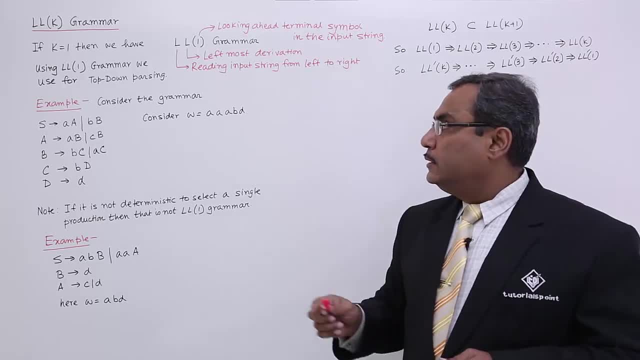 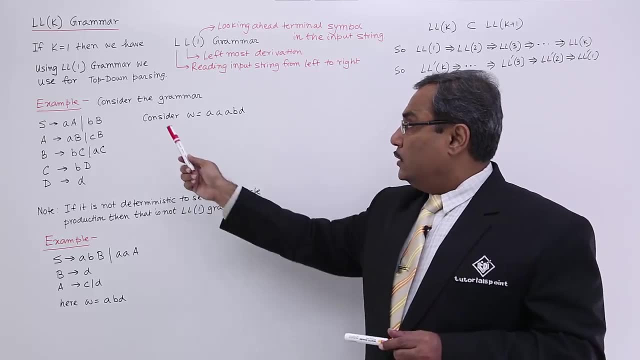 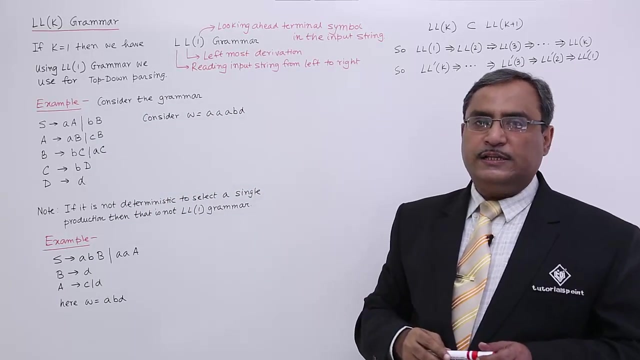 Now let us go of an example that will make our conception clear. Let us suppose when grammar is given- okay, I shall have to tell whether it is LL1 or not. Consider the grammar given and consider this word, that is AAABD, A cubed B, D is my word. 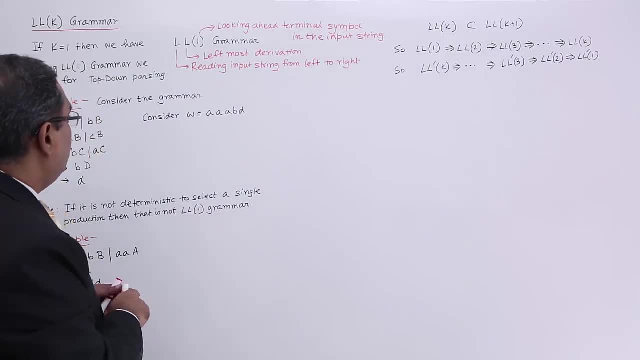 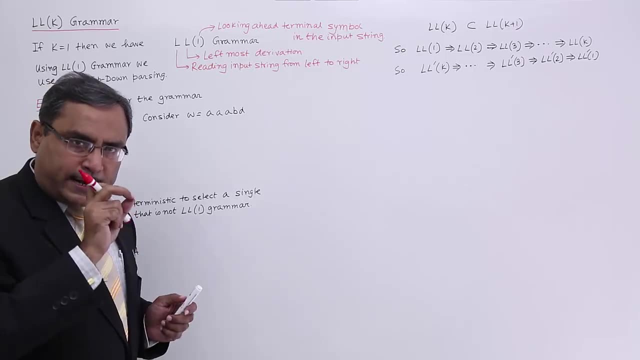 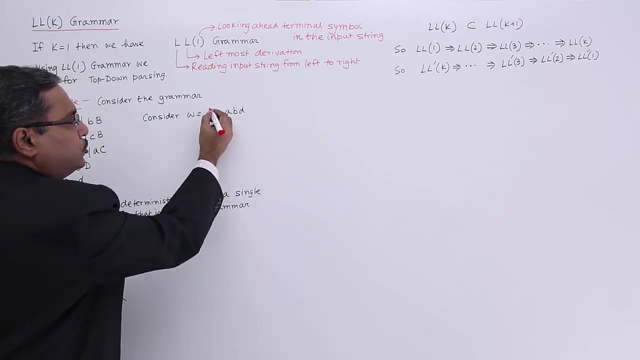 Now let me check whether it is LL1 or not. Okay, Now see what I'm doing. I shall read only one symbol, one input alphabet at a time, from a terminal W. So that is why it is LL1.. And I shall read this one from left to right. So I shall be. 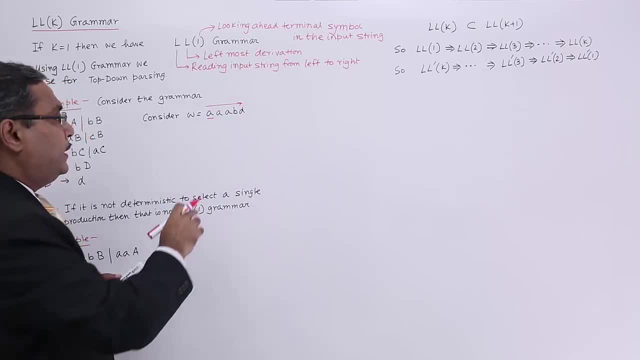 reading this one from left to right, and I shall read one symbol at a time. So my start symbol is S, My start symbol is S, So S I am supposed to make A here, I am supposed to make A here. 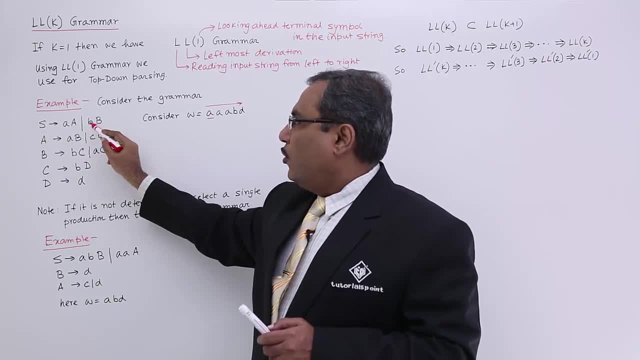 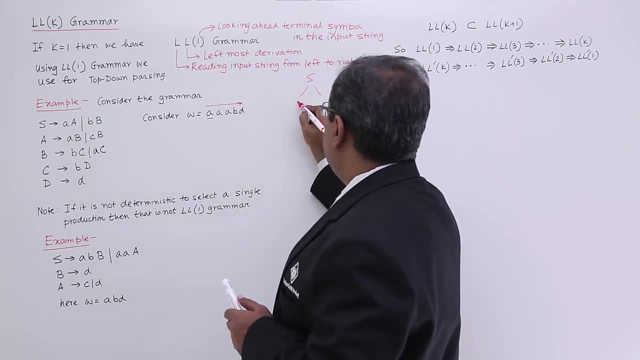 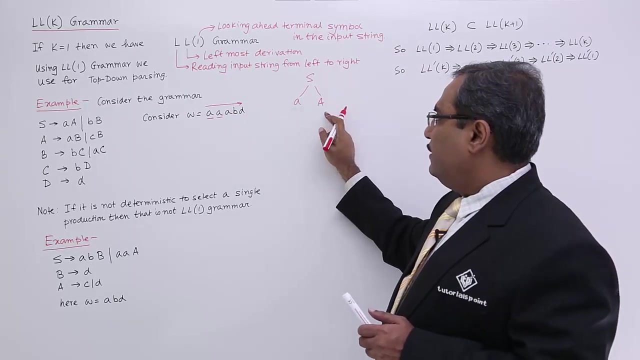 So we are having two options: AA or BB. Obviously, I shall be applying this one. It is deterministic, I can apply this one, So I shall go for. S produces AA, So I have got this A. Next time I shall read this A. So in the leftmost derivation. 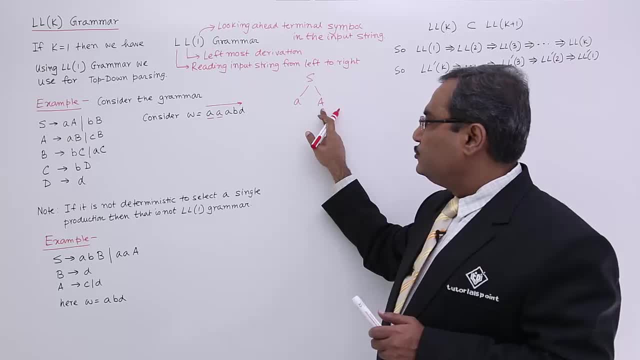 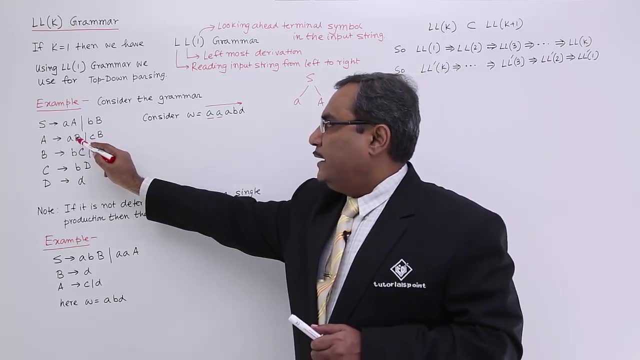 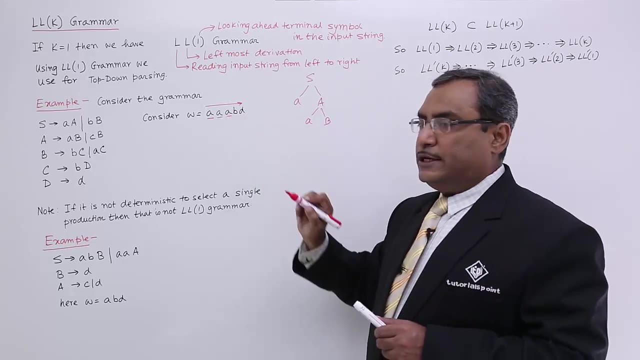 this is my leftmost non-terminal. I am supposed to deduce that one So A. I require A. So which production rule should I use? Obviously, which is starting with A, So I shall make this one as AB. Now, next symbol. I shall read: Look ahead symbol. I shall read: 1. One symbol at a. 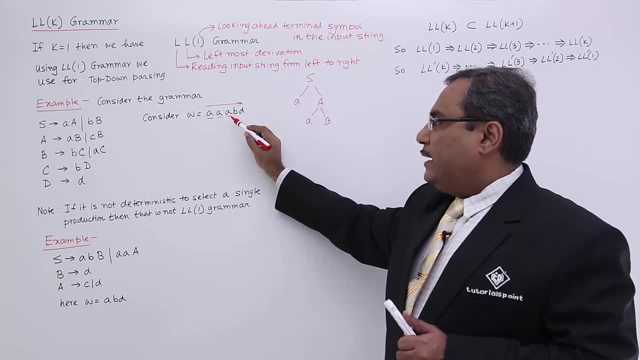 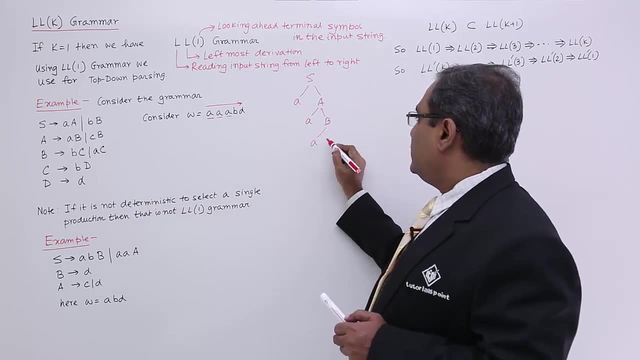 time. So now, B From B. I require A From B. Are you having any option to have A? Yes, I am having. That is A capital C. So from here I shall go for A capital C. The next symbol I want to read is B. So 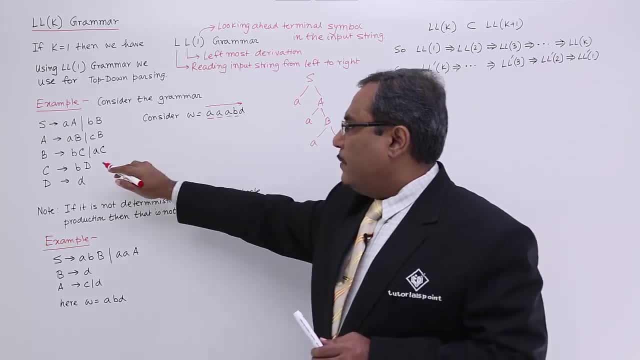 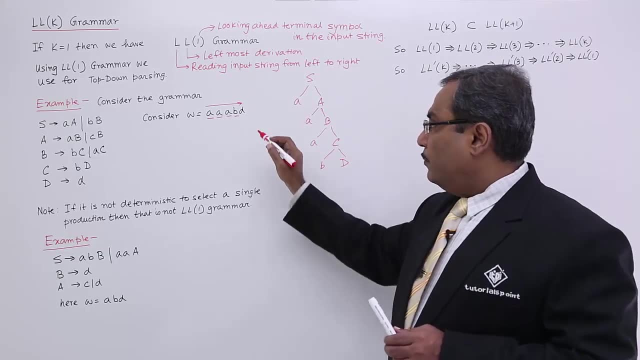 from capital C. are you having any option for B? Yes, I am having one option and that is starting with B, So I shall go for BD From D. can you produce small d? Yes, I am having one option: Small d produces. 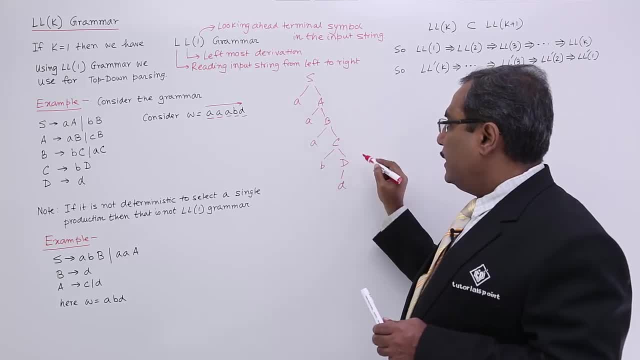 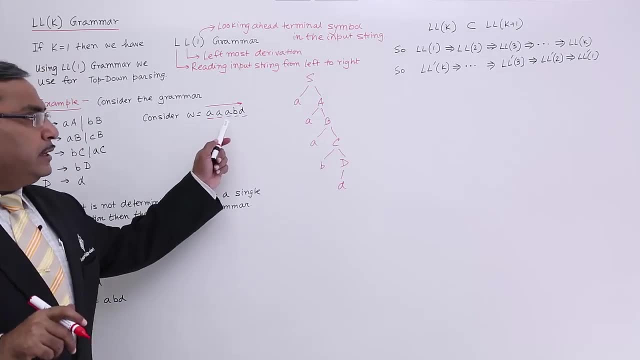 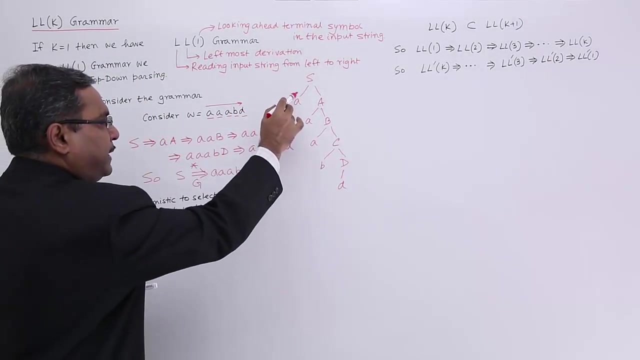 So capital D produces small d, So I can produce that one. So in this way I can derive this particular parse tree. So this derivation tree construction for this particular W indicates that it is LL1 grammar, So it can be expressed in this way also. So this is my explicit. 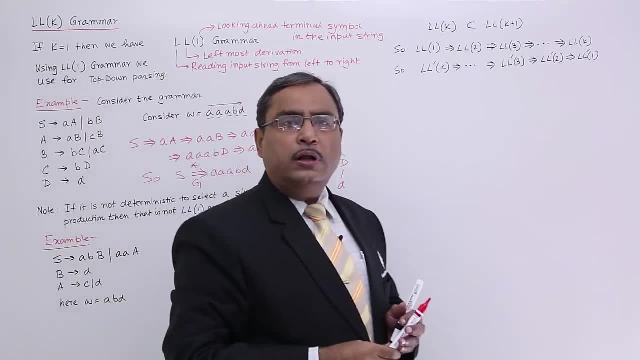 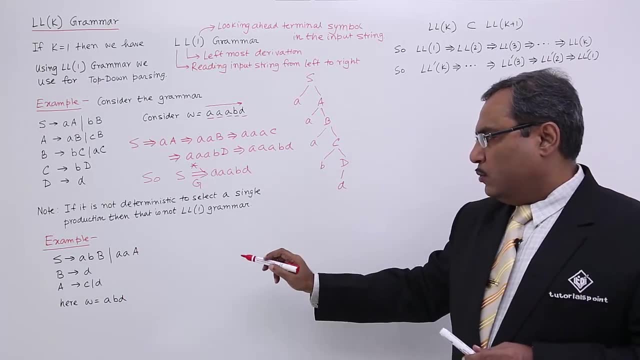 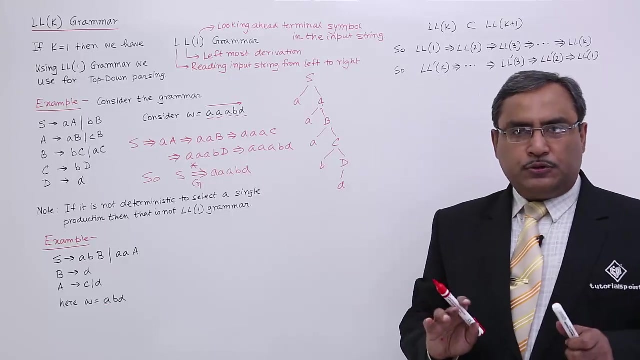 parse tree, and that is my implicit parse tree or derivation tree. So in this way I have done. Now please consider this example. So here we are having one W That is A B D. I want to make A B D, So I am reading this one. Let us suppose that I am supposed. 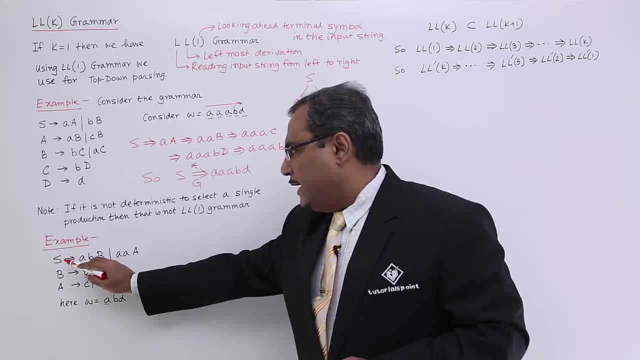 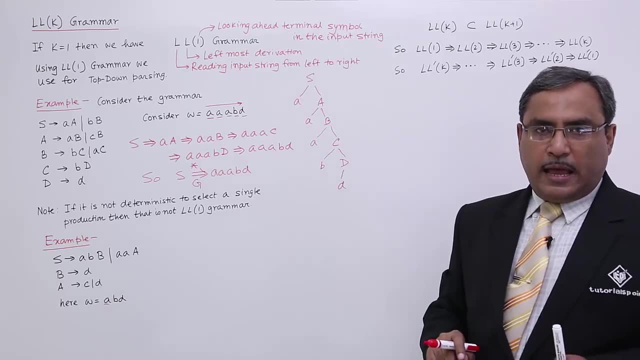 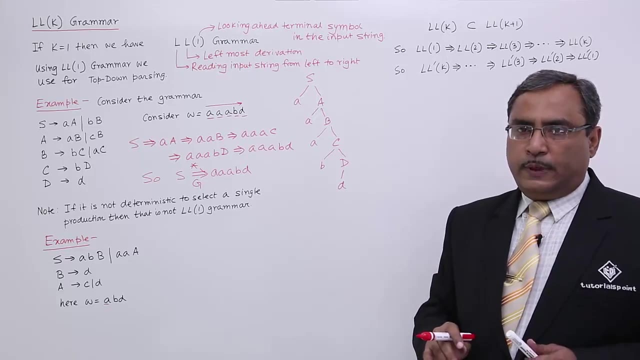 to prove that, whether it is LL1 or not, From S I am having two production rules starting with A, So there is some ambiguities there. Ambiguity means I am not getting the idea that which production rule has to be used, So it is not at all LL1.. So now go for. 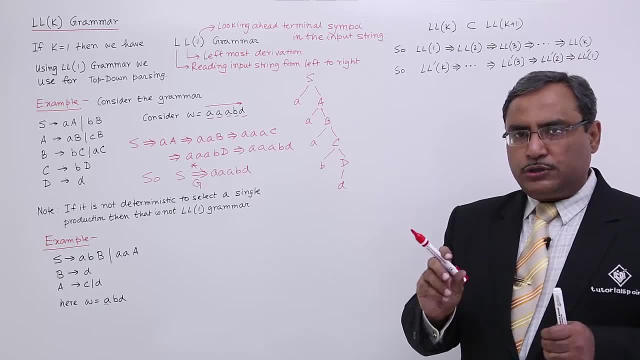 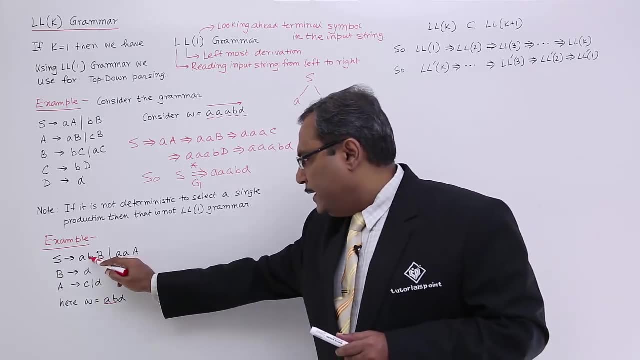 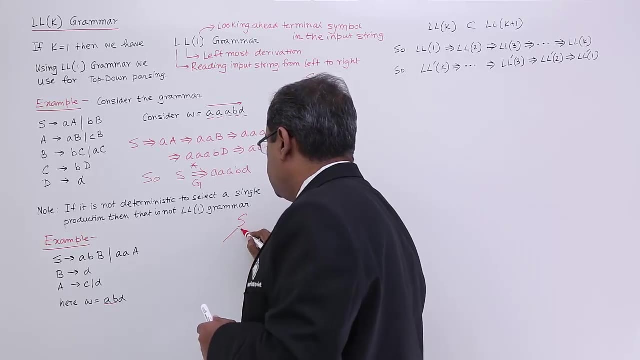 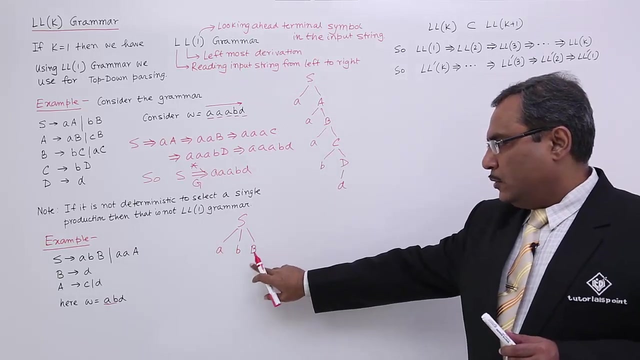 LL2.. So here I shall be reading two symbols from the input. So if I read A B, if I read A B, then are you having any option for producing A B at the front? Yes, I am having this one, So I shall go for S. produces A, B, B Now. so 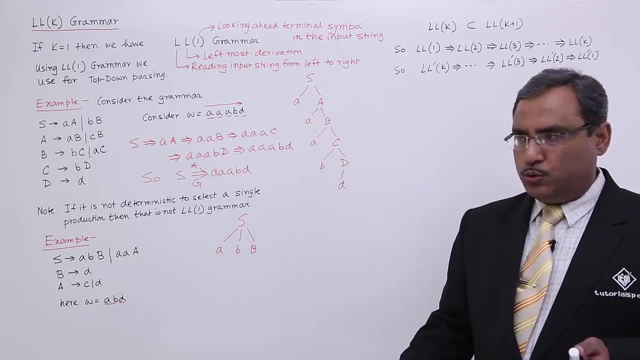 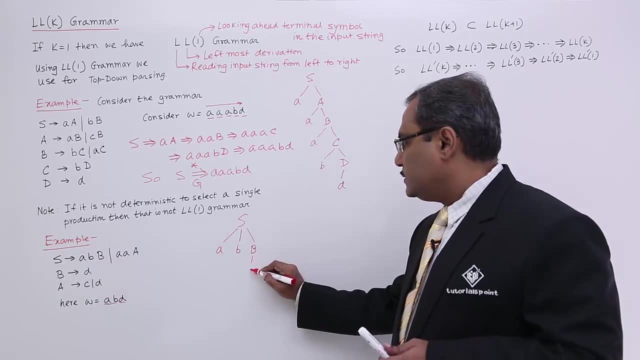 I shall go for another symbol. I am remaining with only one. How can I read two? So I am getting this D From B. is there any option to get D? Yes, that is one option. So I am getting this D, So I shall go for this. So this grammar is not LL1, but LL2.. So 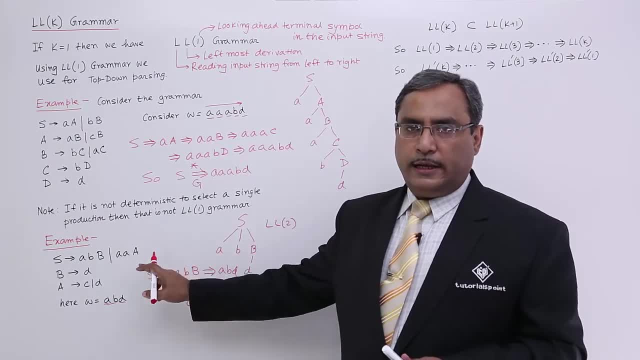 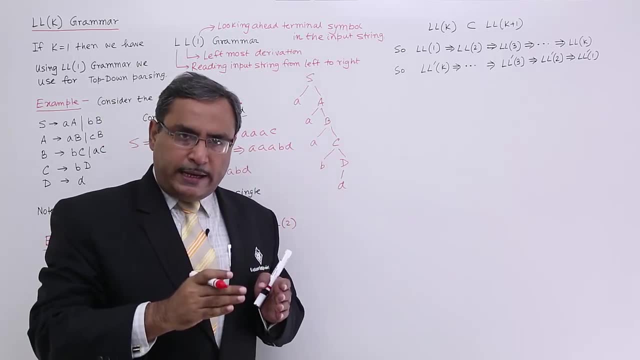 in this way I have proved that it is not LL1, but it is LL2.. Now see, LLk will be a subset of LLk plus 1. If a grammar is satisfiable, or say, if a grammar the parse tree can be. 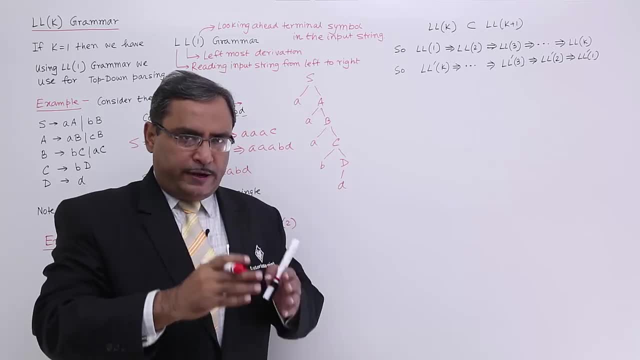 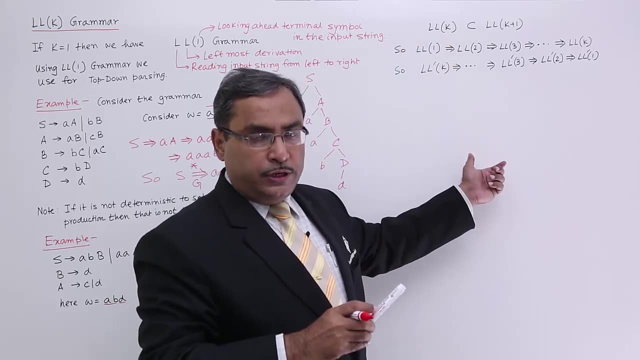 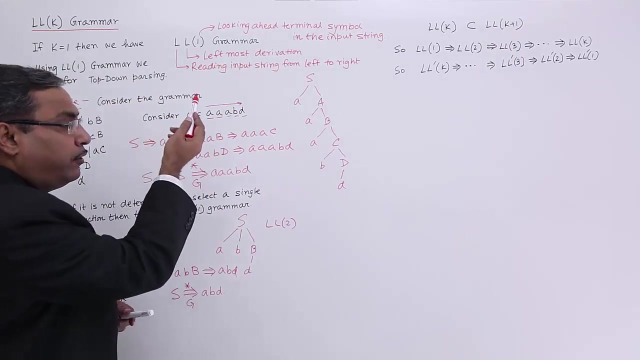 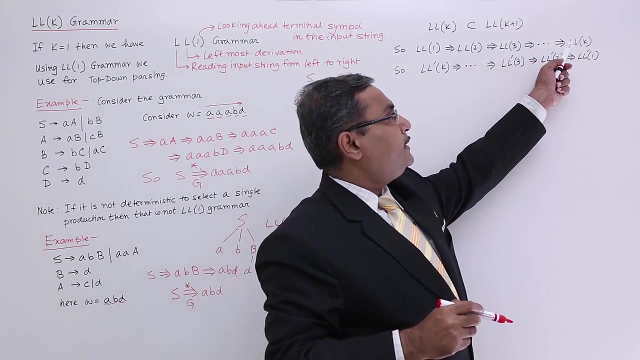 deduced using k sets. So if it is LL1,, then obviously it is also LL2.. So if it is LL1, means it is LL2,, means it is LL3,. dot, dot, dot dot means it is LLk. But if it is not LLk, that means reading k. 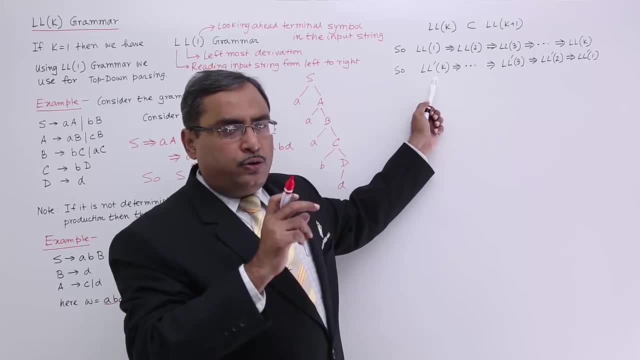 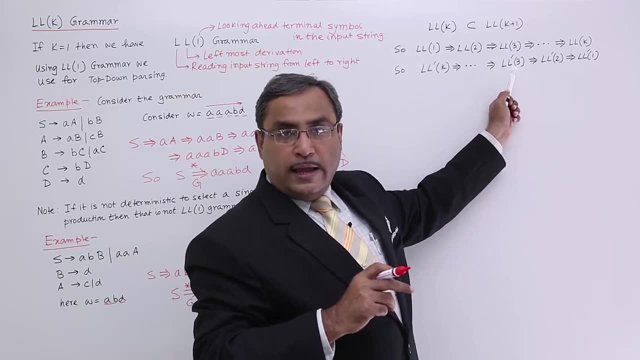 symbols, I cannot read it. So if it is LL1,, then obviously it is also LL2.. So if it is LL0,, choose the null and resolve the ambiguity. I do not know that which the poor clap is to be used. so if it is no, So that means it is also not LL3, not LL2, not LL1. So 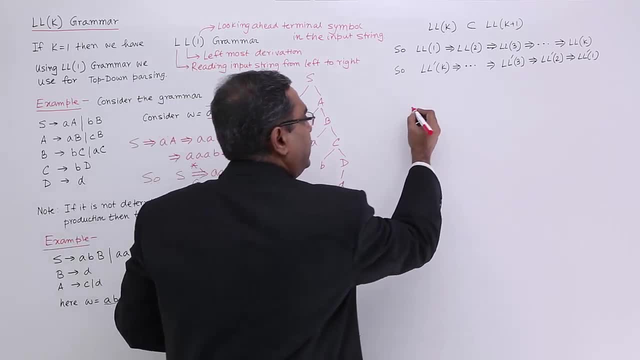 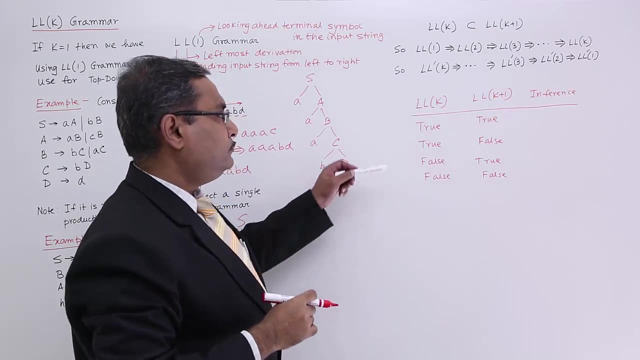 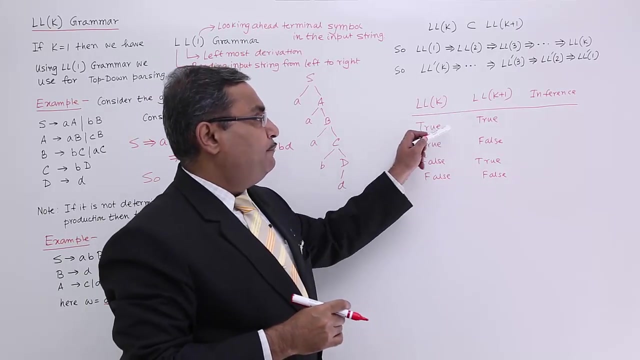 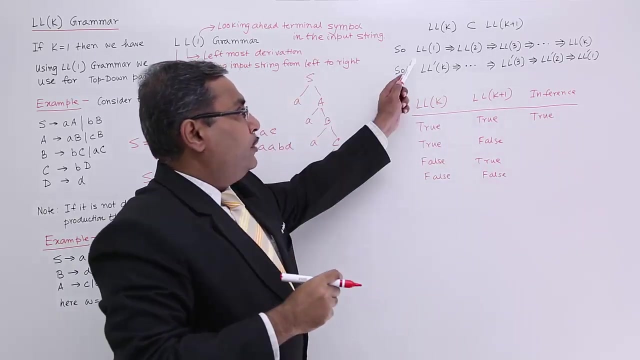 in this way I have written. Now let me consider one thing. Say one grammar is LLk. Okay, I am writing at first. Okay, Now say a grammar is LLk and the grammar is LL3.. So k plus 1. if both are true, that means it is true. yes, it can happen, because already you. 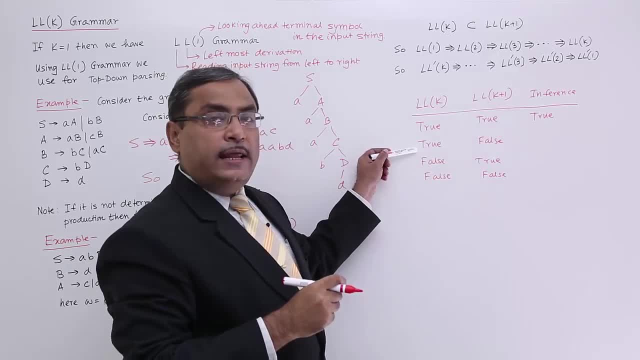 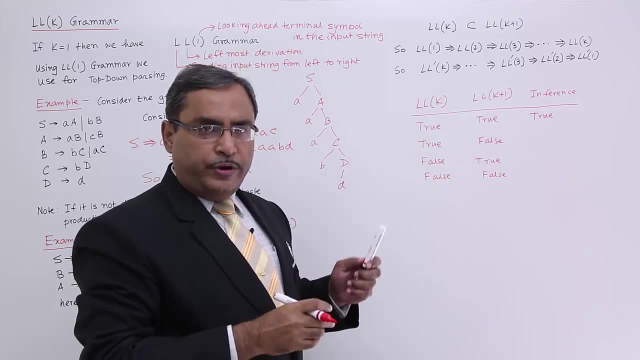 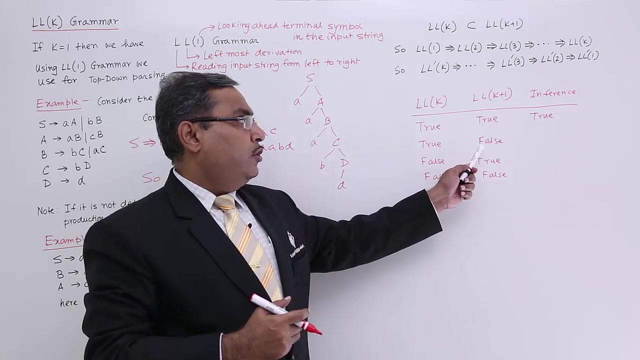 have written that one. if the grammar is l, l k but the grammar is not l, l k plus 1, it cannot happen because reading k number of symbols from the input string from the left, if you can deduce the first string without any problem, then obviously with the k plus. 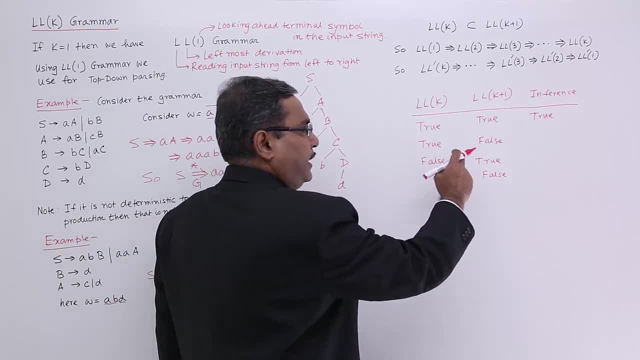 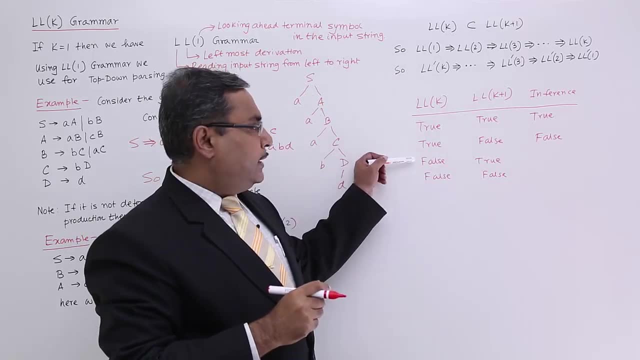 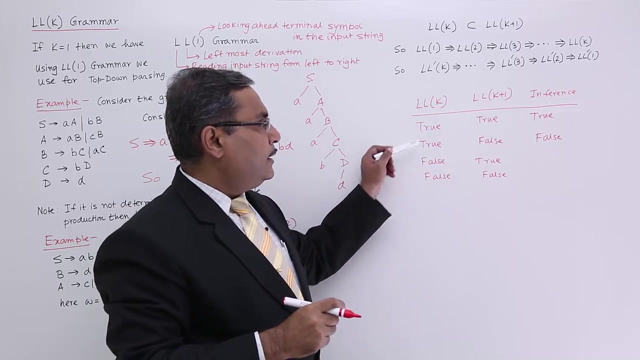 1. look ahead symbols. obviously there should not be any problem. so if it is true and if it is false, it is false. if the grammar is not l l k, then the grammar is not l l k plus 1. also, so sorry. if the grammar is not l l k, the grammar is l l k plus 1. true can be. 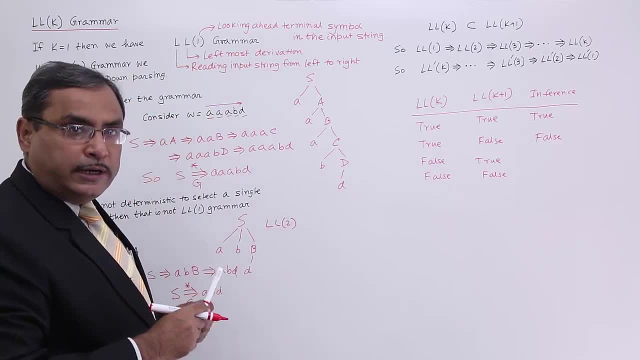 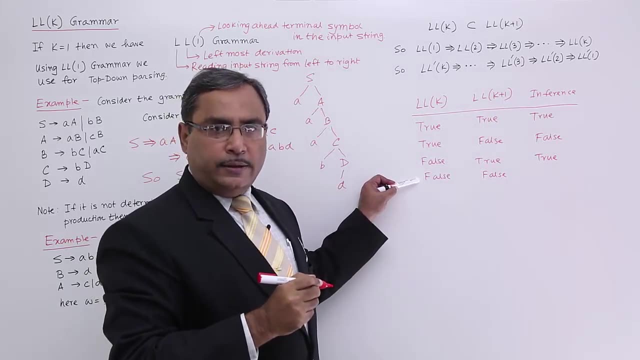 because here you see, this grammar was not l l 1, but it is l l 2, so it is. it can happen this one: if the grammar is not l l k, that the grammar cannot be l l k plus 1, so that that can be.